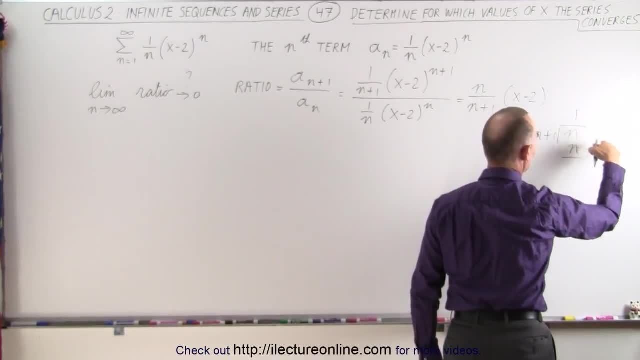 n plus 1 is n plus 1. when we subtract, we get 0 minus 1, which is minus 1.. so that means that n divided by n plus 1 can be written as n minus 1 over n plus 1.. so let's do that instead, because 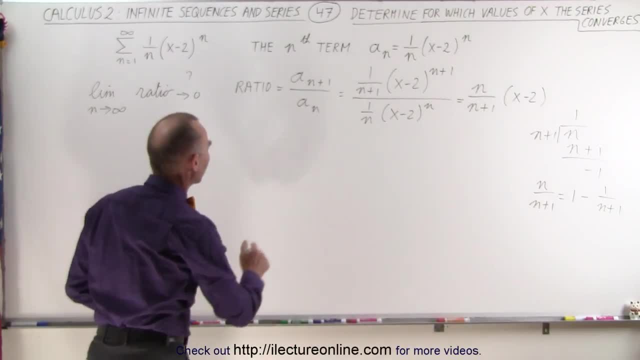 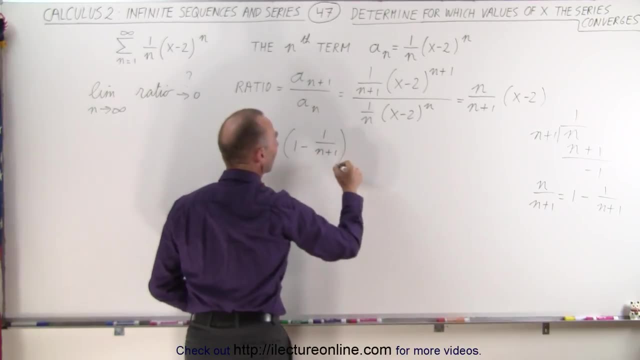 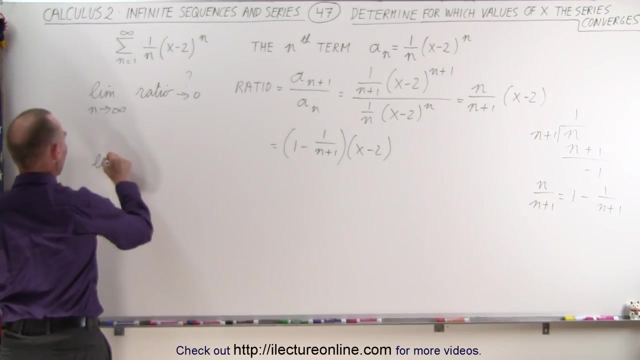 it makes it easier to find the limit. so the ratio is then going to be equal to the quantity 1 minus 1 over n plus 1, multiplied times x minus 2. and now we're going to take the limit, the limit as n goes to infinity- of 1 minus 1 over n plus 1. 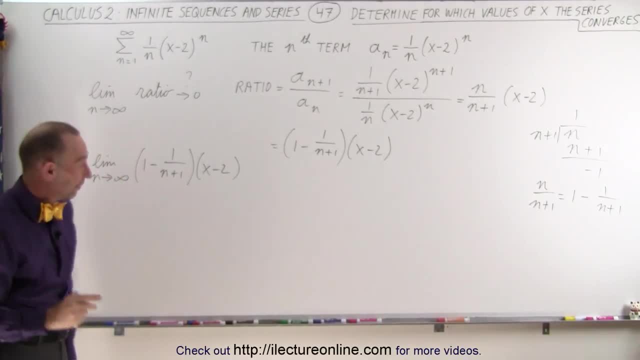 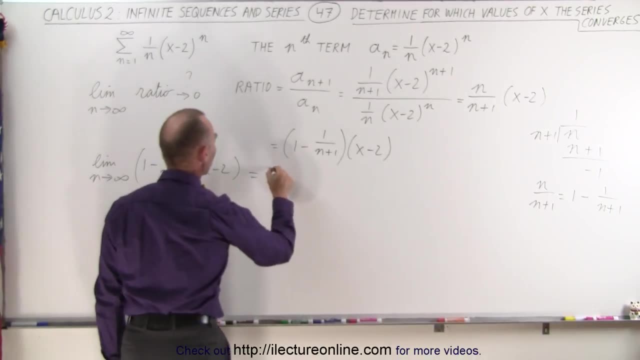 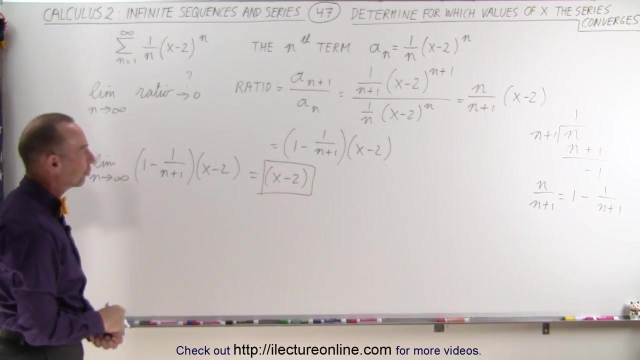 times x minus 2.. so when n goes to infinity, 1 over n plus 1, well, this will go to 0, and so then we end up with 1 times this or x minus 2.. so in the limit we see that the terms will converge down to x minus. 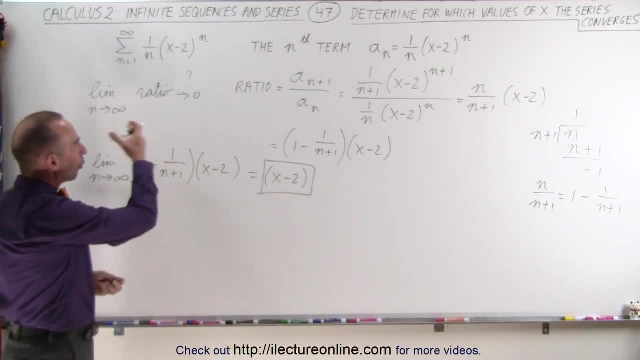 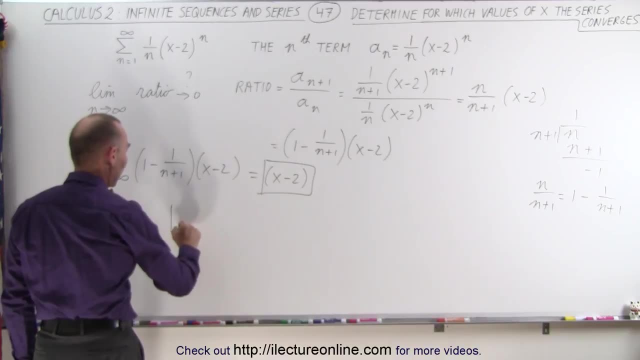 2.. so for which values will the whole series converge? well, that is. the necessary condition, then, is that the absolute value of x minus 2 must be less than 1. and we can solve that by saying: that means, therefore, when this is a positive value. 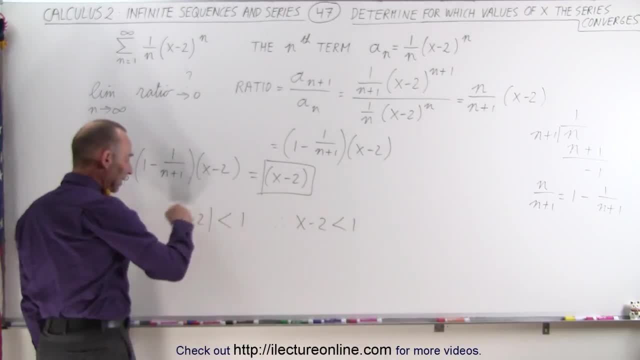 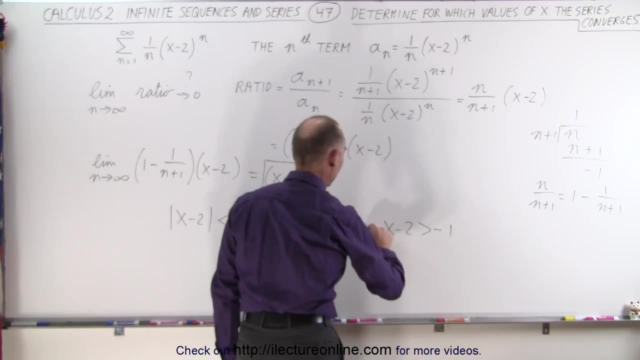 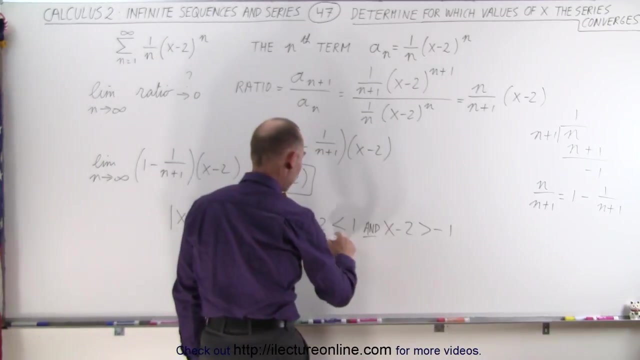 x minus 2 must be less than 1, and if this is a negative value, then we could say that x minus 2 must be greater than negative 1, and that must be an and condition. both of these must be true. that's the case. we then say that when we bring the 2 across, we get x must be less than 3 and 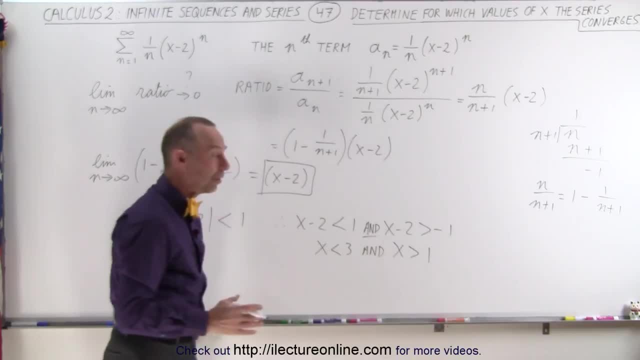 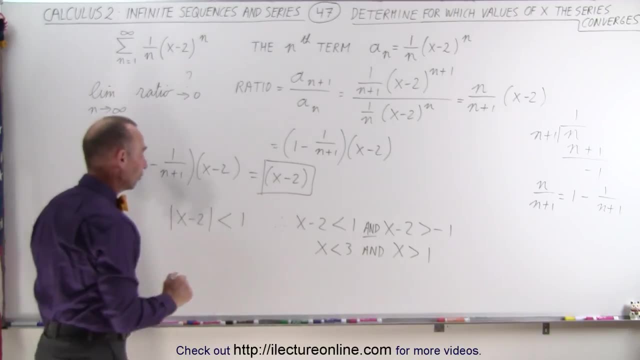 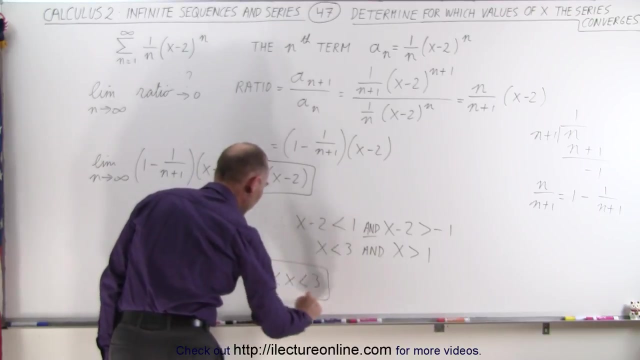 x must be greater than 1, which means that only if the value of x is between 1 and 3, then this series will converge. so therefore, we know that 1 must be less than x, which must be less than 3, and for that range between 1 and 3. 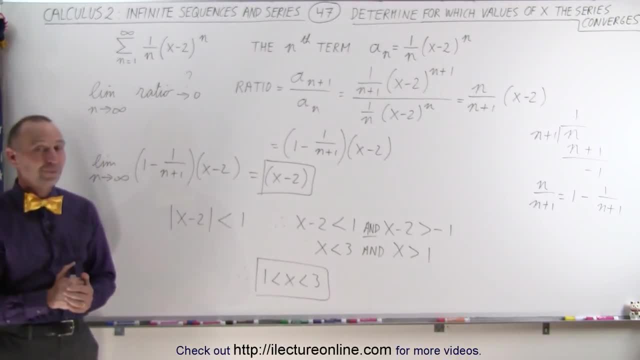 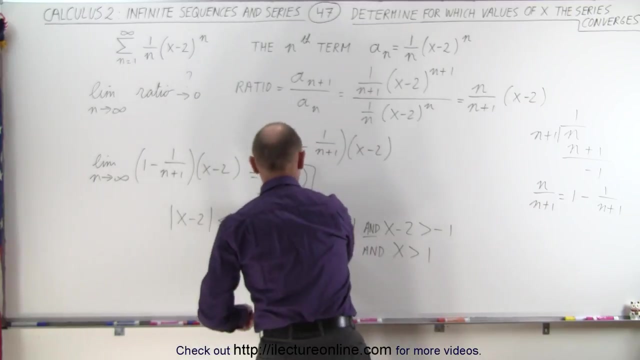 for those value of x. this series will indeed converge. and one more note: we can also solve for something like this in the following fashion. what we can do is we can simply place this value between the negative and positive value of 1, and so this can then be also solved.